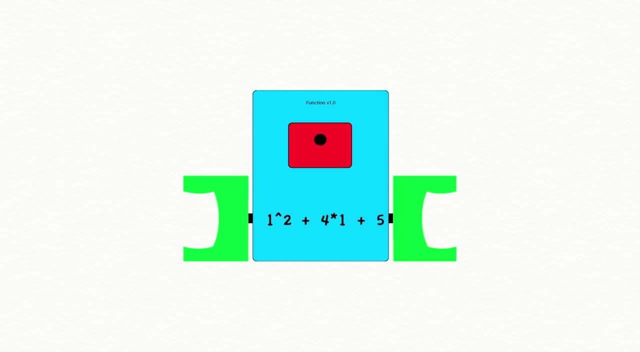 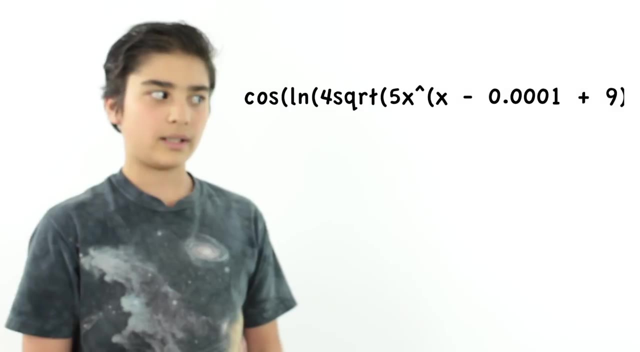 then take that original number and multiply it by 4. You take those new two numbers you calculated, add them together and add it to 5.. It's a little bit more complicated. I don't even want to look at that one. These equations allow you to mathematically figure out. 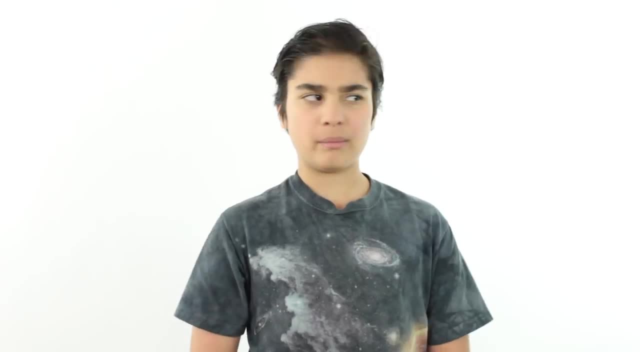 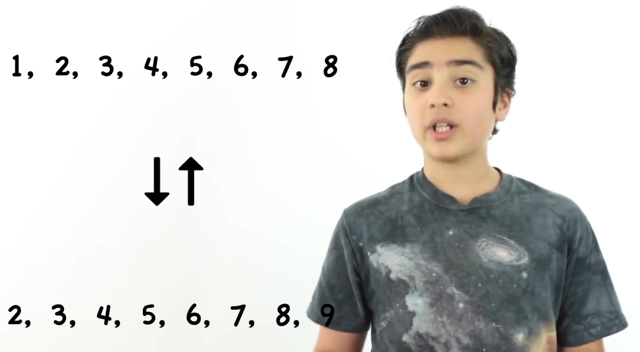 which outputs you get from the input that you put in. But what do they have to do with graphs? Well, let's see If we get a bunch of inputs and figure out their outputs and pair them up. we have a bunch of plot points. 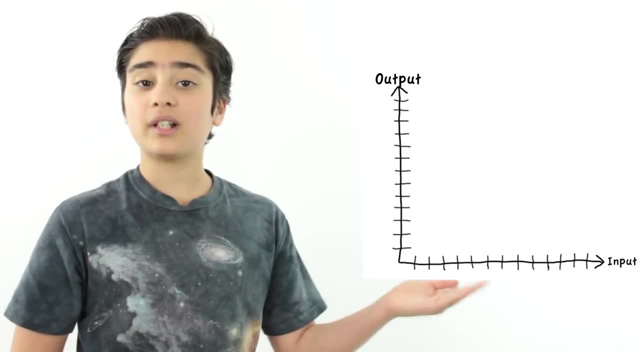 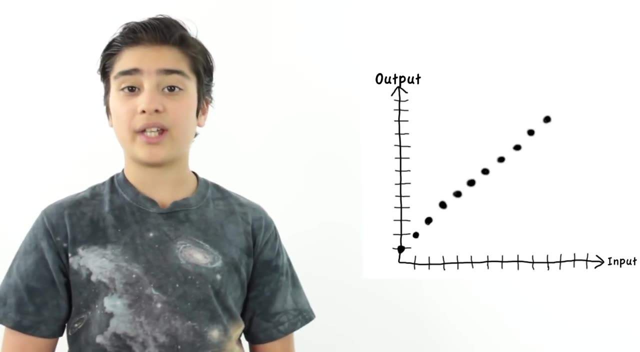 Let's say we have a graph like this one. Let's say, the horizontal line describes the numbers you put in and the vertical line describes the numbers you get out. Now you can use these plot points that we calculated and put them on this graph. 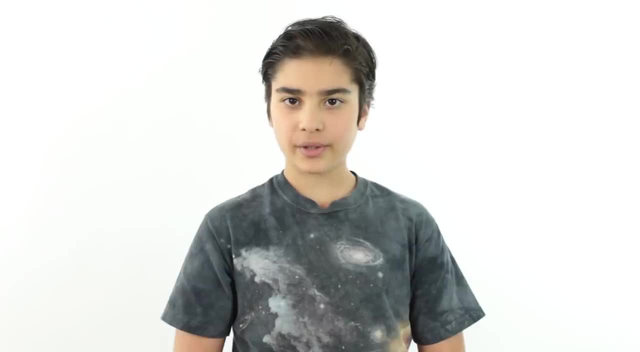 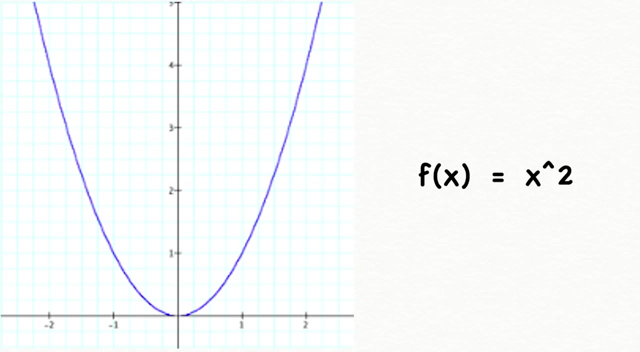 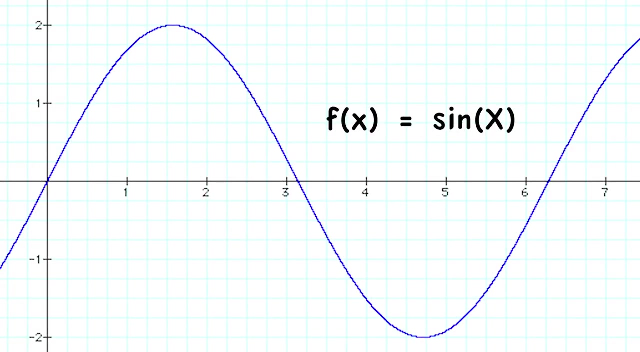 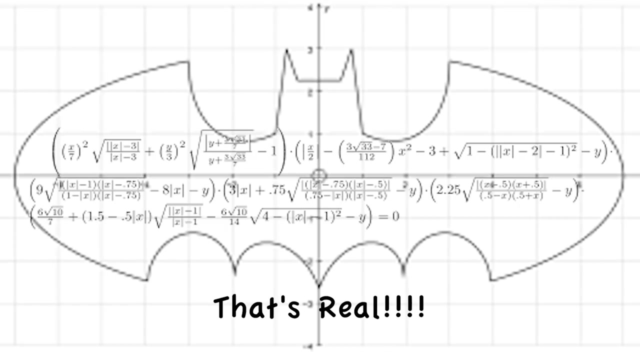 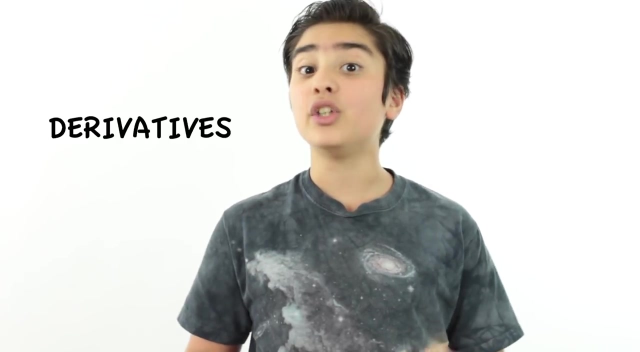 Now, if we do connect the dots, there's our graph. We can create a graph for any function. Check these out. These functions are great, but they're not very good at identifying change over time. That's where calculus, specifically derivatives, come in. 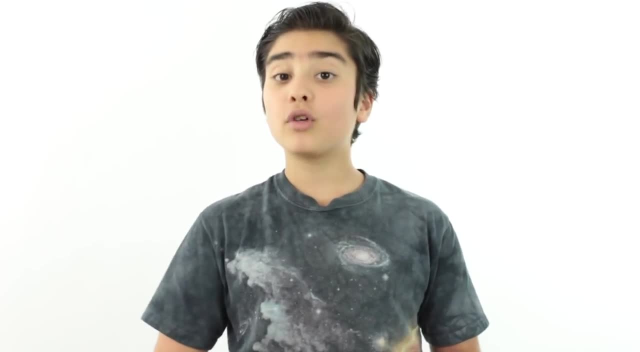 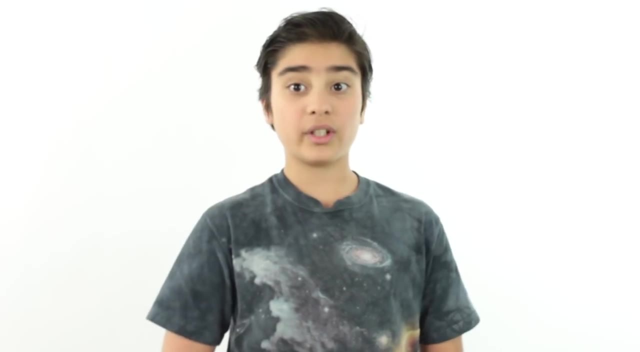 Derivatives allow you to see how something changes. So if we call the original function f of x, then we can call the derivative f, prime of x, which is basically just adding an apostrophe. So you can find the derivative with the equation. 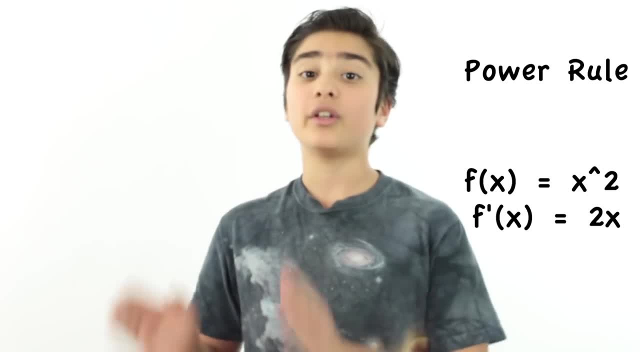 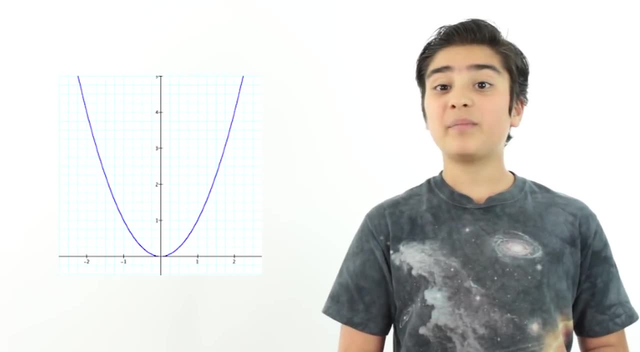 using something called the power rule, or you can find it on the graph With something called the slope of the tangent line. Let's take this graph over here of x squared. The tangent line is basically a line that just barely touches the graph. 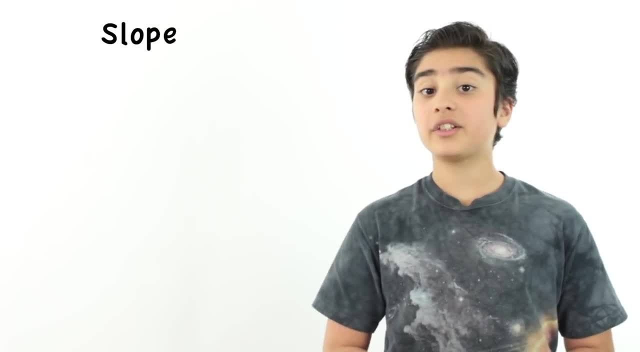 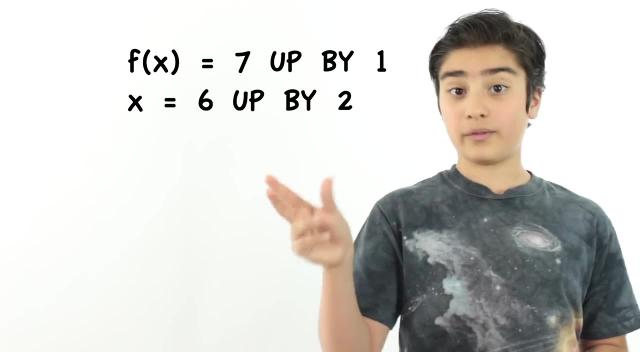 Like this one right over here, And the slope allows you to determine how much something increases over a period. So, for example, if the value of a function increases by one over a period of two, the slope becomes one over two or one half. 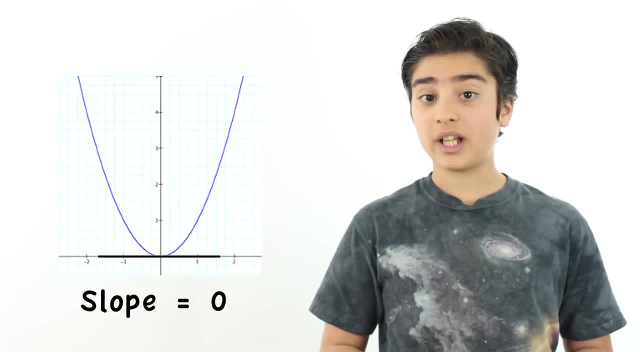 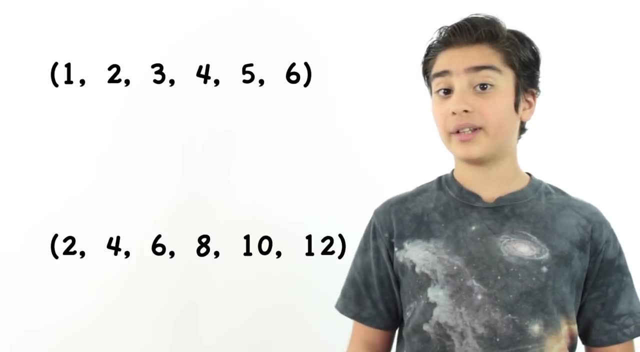 At this very point on the graph, the slope of the tangent line is zero. So if we were to find a function with a slope of the tangent line on every point on this graph and then create plot points out of those and connect the dots, 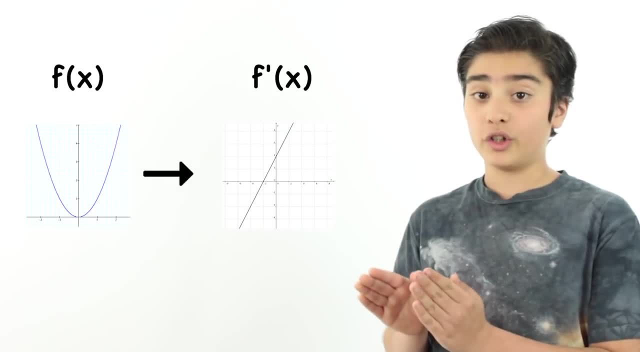 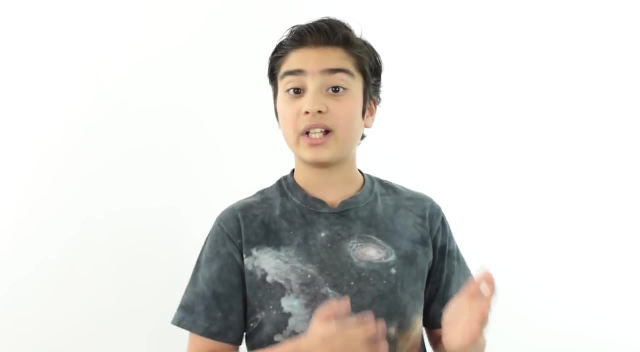 you would have the graph of the derivative of this function. Okay, so we explained derivatives. they're all fancy and such, but what's the use in real life? This is where we come back to Isaac Newton. Newton was studying physics, specifically velocity and acceleration. 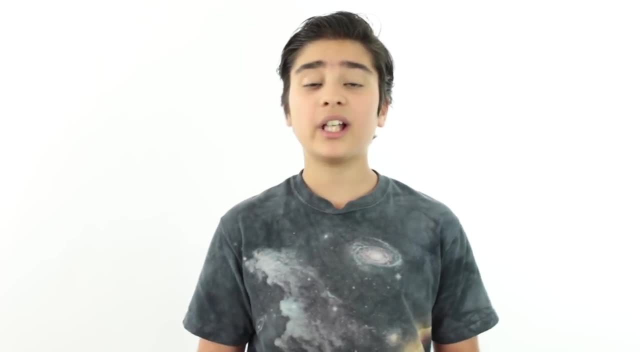 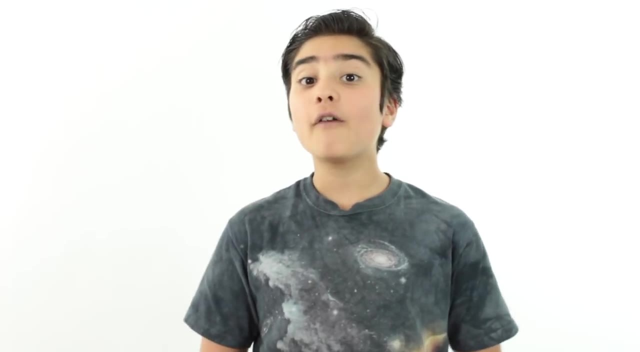 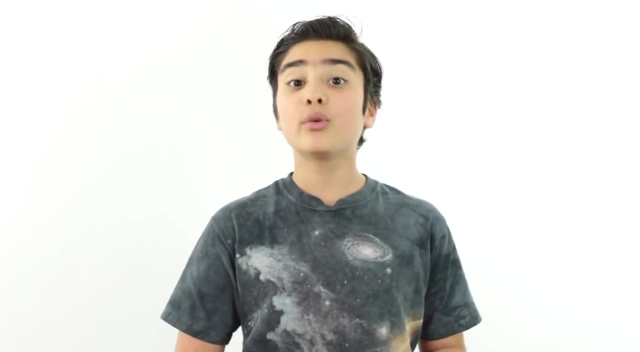 Velocity measures the speed at which you're traveling. Acceleration measures how fast your speed is increasing. In other words, acceleration is describing how velocity is changing. But Isaac Newton didn't have terms like derivative or calculus in the past. He needed to figure out the relationship. 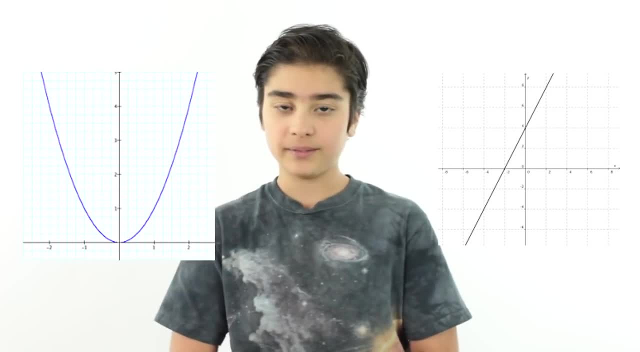 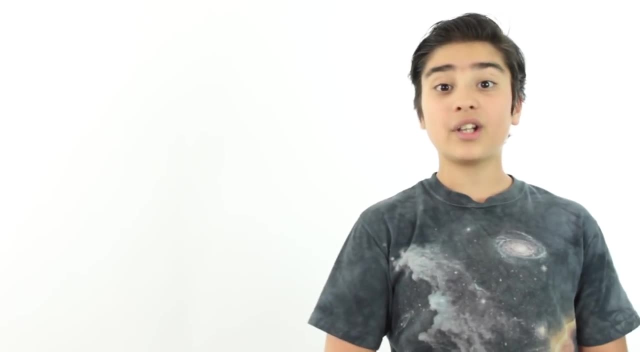 between the graph of the acceleration and the graph of the velocity. We hope you enjoyed this video. Stay tuned for our next two videos. Subscribe to us over here or check out one of our other videos over here. And, as always, science is everywhere. and in everything Bye. 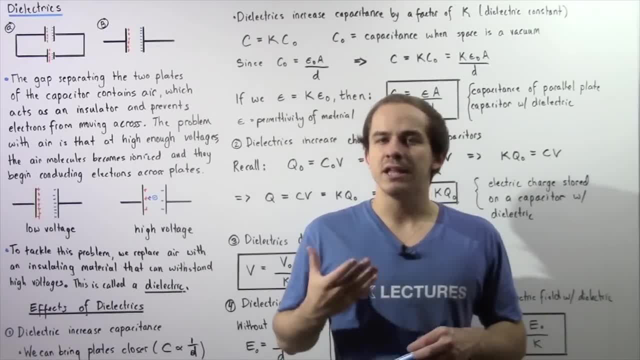 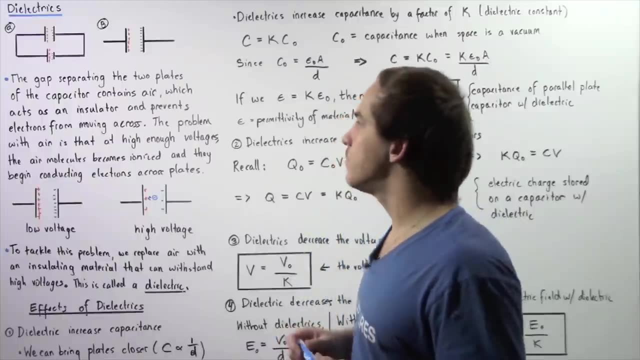 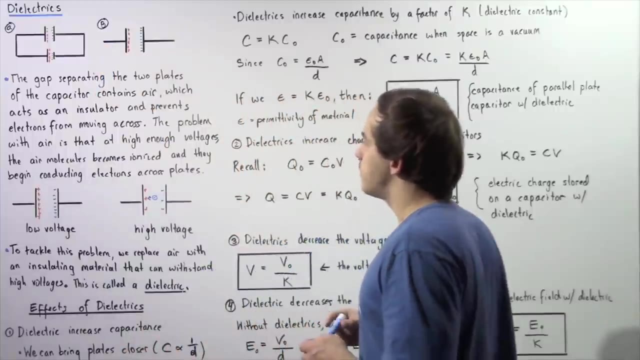 Capacitors are very useful devices as they allow us to store electric potential energy within the electric field that is created as a result of a separation of electric charge. So let's begin by looking at these two diagrams that have parallel plate capacitors. So in diagram A we have a parallel plate capacitor and we also have a battery. 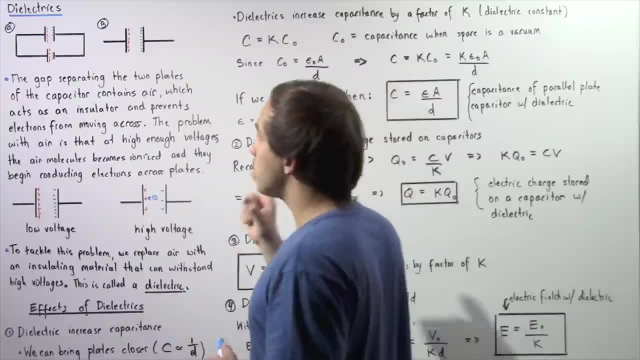 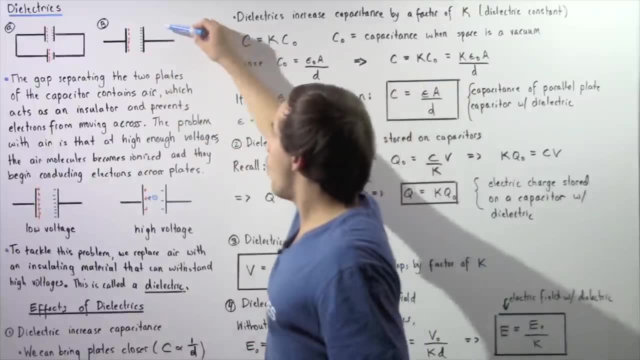 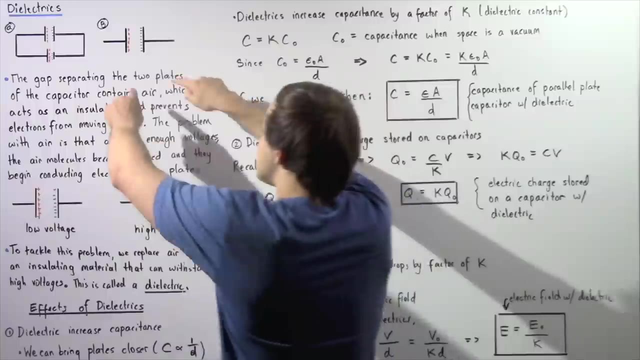 Now the battery essentially acts to charge our parallel plate capacitor, And when that capacitor is fully charged it looks something like this: So one of the plates has a negative charge. the other plate has a positive charge. Now, because they are separated by a certain distance, that means we have a separation of electric charge. 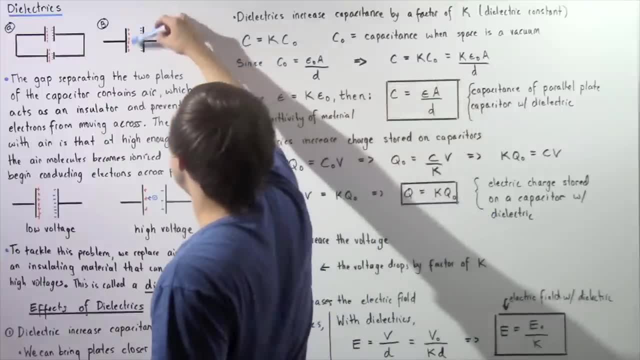 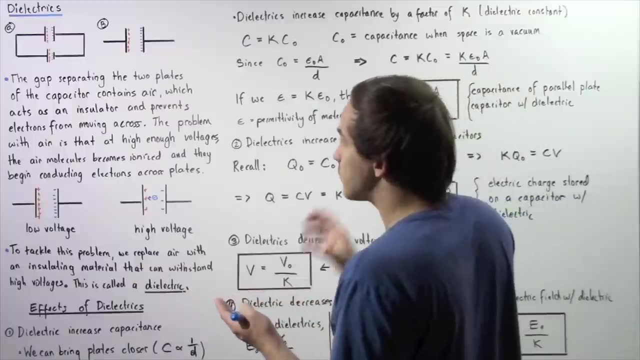 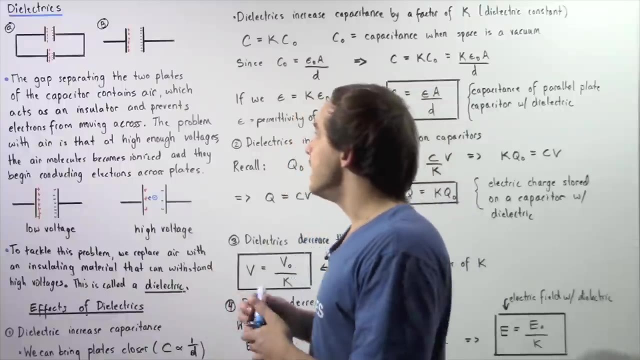 and that will create an electric field midway or in between our two plates, And we can then store electric, potential energy, within that electric field, Which then can be used to do useful work, for example power a computer or a phone. Now, the gap separating the two plates of the capacitor contains air.